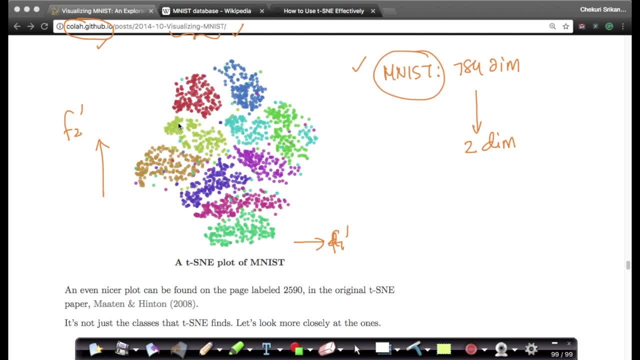 Okay, Now comes the interesting part. So, since we've understood this, so there is one aspect that I wanted to go over. So all these are zeros, right, But I have one point here which is actually five, because these light blue colored points are my fives. So there is one five here. But if you 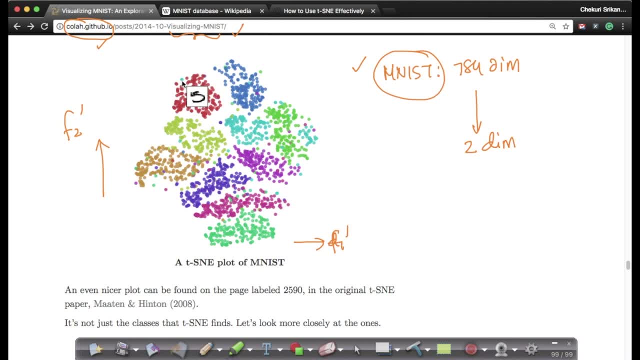 notice that five as I'm hovering my mouse around it, that five looks very much, very close to a zero. That's why it was grouped together with zeros. Okay, From this plot, we cannot interpret that. okay, that the spread is zero. So we cannot interpret that. okay, that the spread is zero. 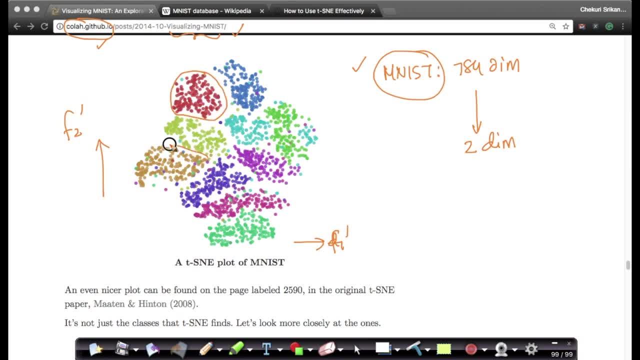 So the spread of that. zeros are here, ones are here. Okay, We cannot interpret, we cannot interpret. we cannot interpret cluster sizes, cluster sizes or inter-cluster distances or inter-cluster distances in t-SNE, right. So we saw this when we were going through the 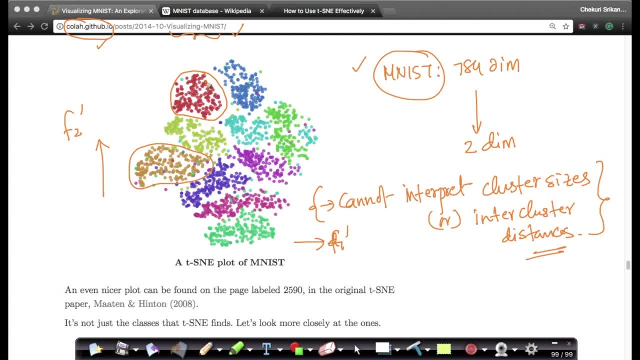 distalpub examples. right? So we saw this when we were going through the distalpub examples, right? So we saw this when we were going through the distalpub examples, right? So I cannot say that, okay, zeros are well spread and so are my ones, So are my. I think these are sixes, or 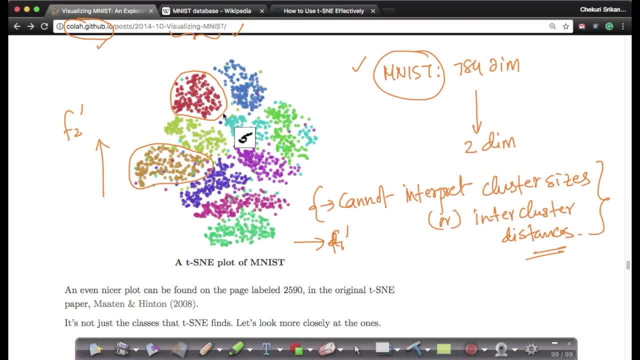 fives right. These are my sixes right, So my sixes are also well spread. I cannot talk about how well spread the points are, So I cannot interpret the cluster sizes or the cluster distances. Suppose if this is one cluster and this is another cluster. I can't interpret this. 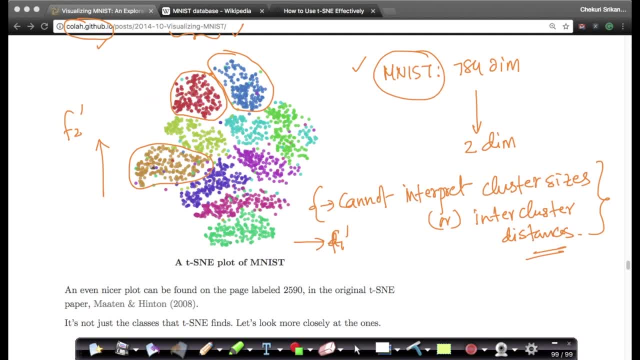 distance. There is no way I can interpret it. Okay, So you cannot interpret cluster sizes and inter-cluster distances from the previous one. So I cannot interpret the cluster sizes or inter-cluster distances. So I cannot interpret the cluster sizes or inter-cluster distances from the previous. 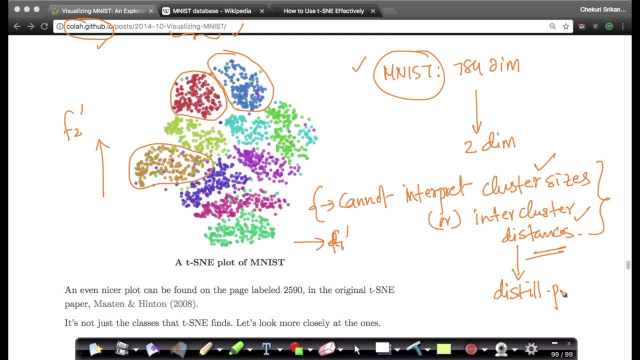 video where we where we saw how to interpret TCNE outcomes, which we saw from distalpub website channel. but here the most important takeaway is that, yes, TCNE in the high dimensional dataset. since I can't visualiza784 dimensions, I have two-dimensional statistics and when visualizing this two-dimensional 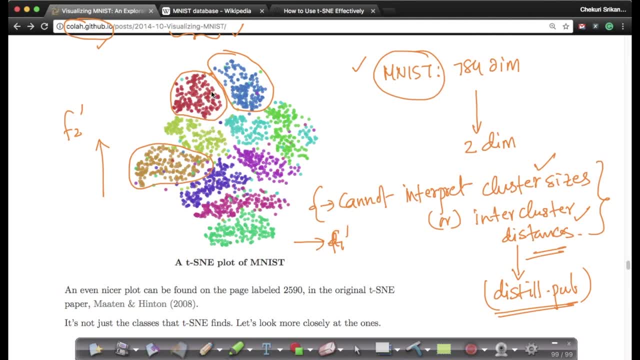 statistics and when visualizing this two-dimension data, first thing I notice is all of my zeros are grouped together. All of my sixes are grouped together Here. if you see your fives, you have a bunch of fives here and you also have a bunch of five. 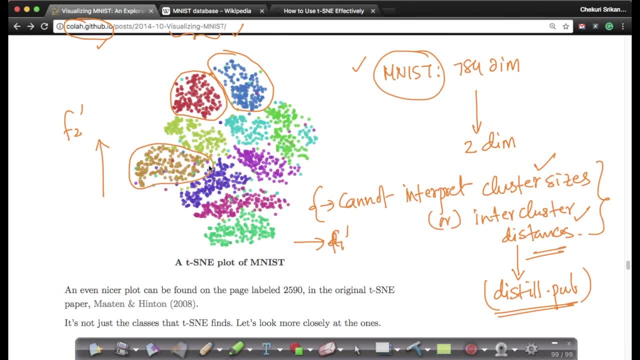 is here. okay, now let's look at once, because once are spread like this. so how do a one somewhere here in this region looks like a slant one? if you see as I'm moving and as I move farther and farther away, inside my one becomes straighter. 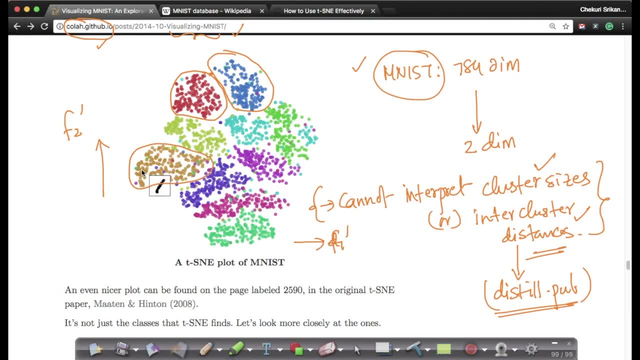 and straighter, or this has become eight already, right. so as I move so here, my once in this region are slant as I'm moving this in this direction. my once as I reach here have become straight line once. okay, so it is not just preserving all the ones, it's also putting ones which are written similarly close to. 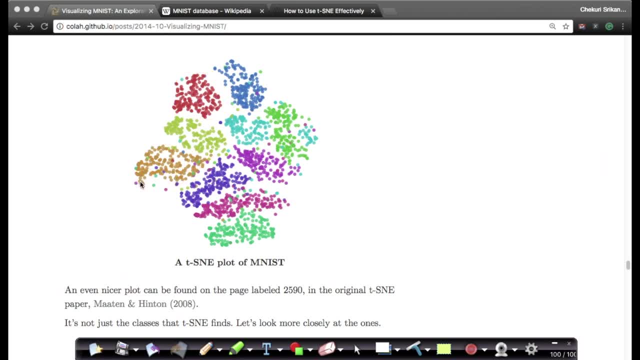 each other right. so let's again see that once more. so the ones that you see here are all slant right. the ones as you're going away become straighter and straighter, which means it's not only separating all of your ones from rest of your characters, but also it's separating all of your slant ones in this region. 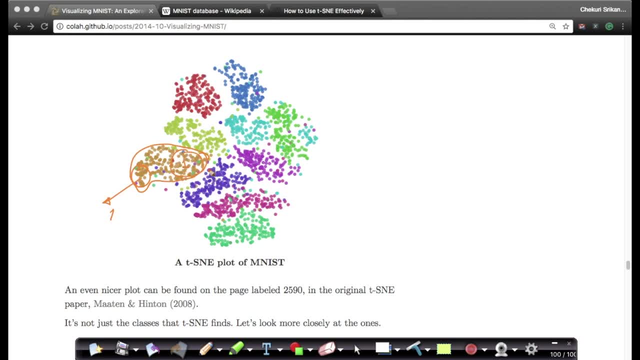 all of your straight ones in this region, all of your straight ones in this region, which is important. right, which means, whatever visually look similar, are getting grouped based on visual similarity, which is extremely important. even similarly right this five: look more like this file. look like this right this. 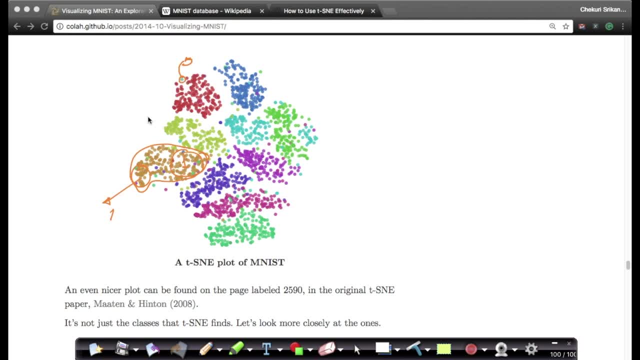 file. look like this, right, let me, let me just change my okay, this five. look like that, right, which is very similar to zero, and that's why it got grouped with zeros. so what my t-SNE, what t-SNE is achieving very successfully, is it's saying that I. 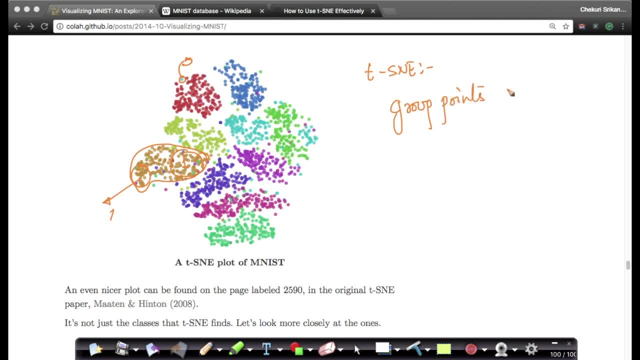 will group points or I will cluster points based on the visual similarity, based on their visual similarity, which is very, very interesting. now, using t-SNE, I have visualized a 784 dimensional data set by embedding this data set into a 2d space successfully, and the big lesson I learned is: yes, points which are visually.